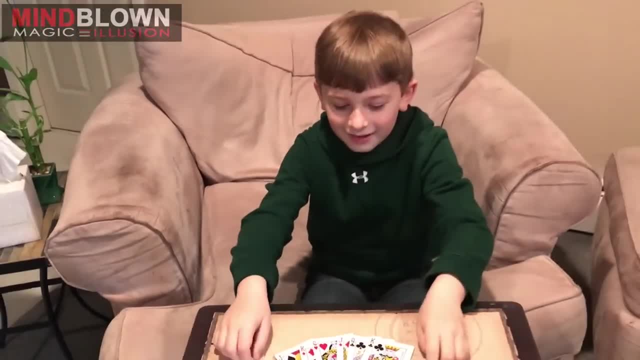 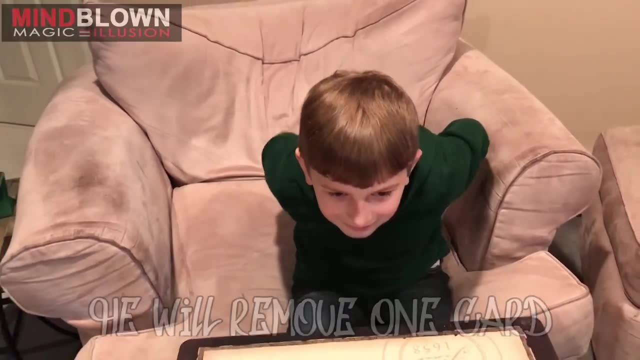 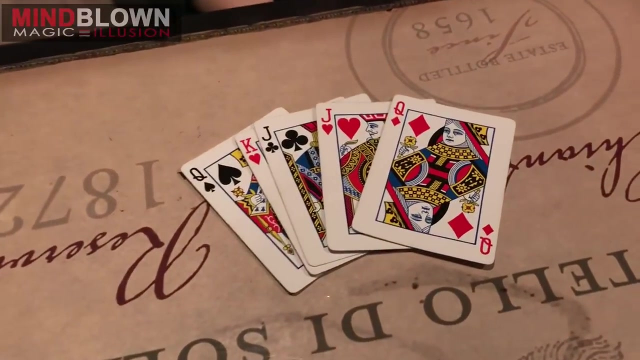 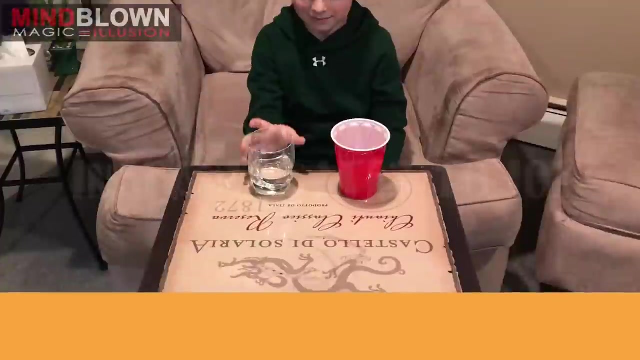 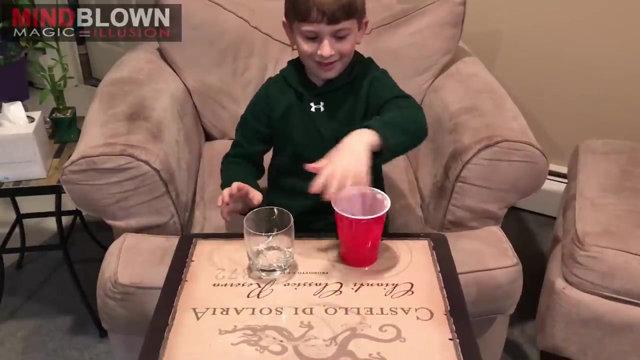 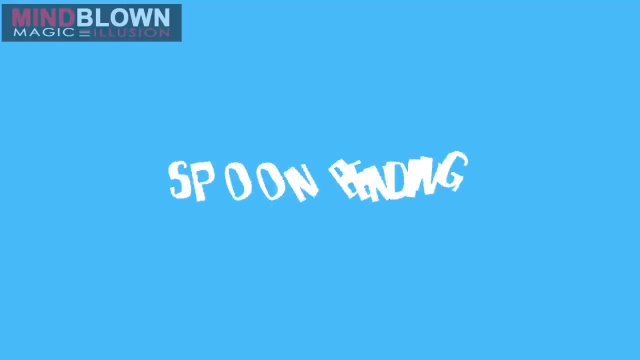 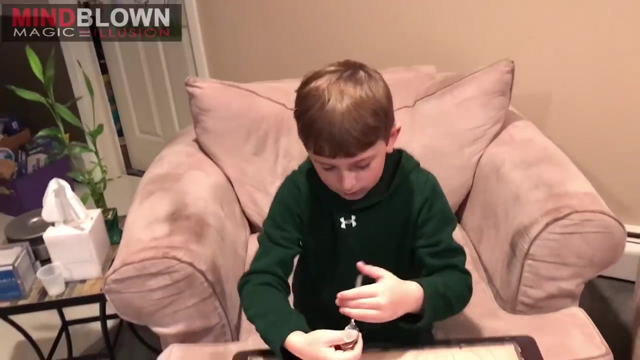 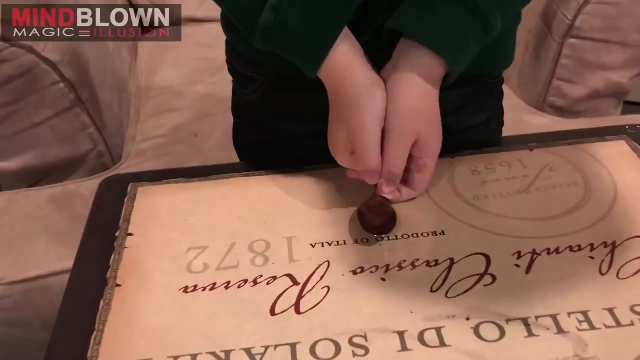 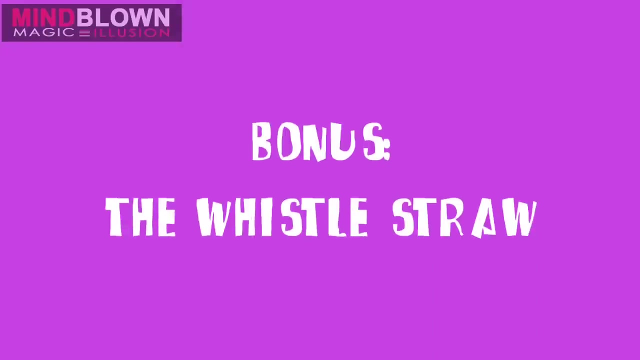 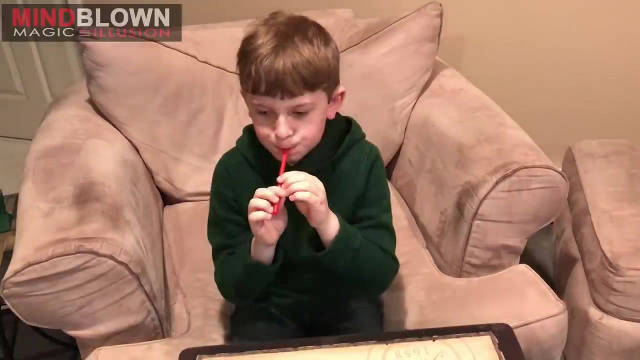 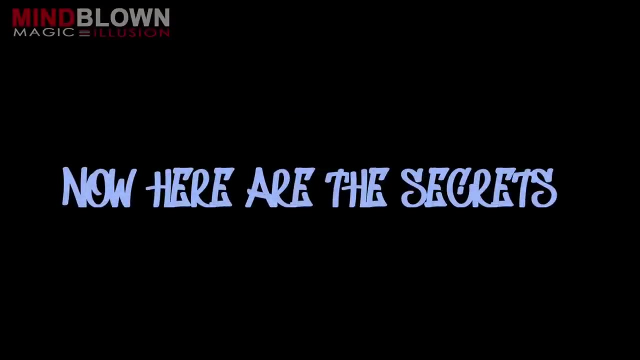 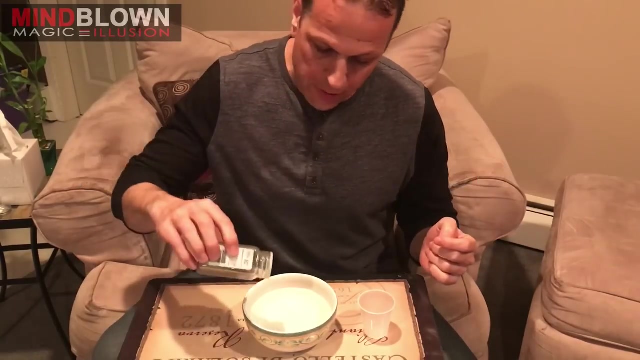 You got it. Okay, now I'm going to take the cards, put them behind my back and remove one. Did I guess your card? Yes, you did. What's great about this trick is that it is completely self-working. You're going to pour the pepper into the water, as you saw him doing the trick. 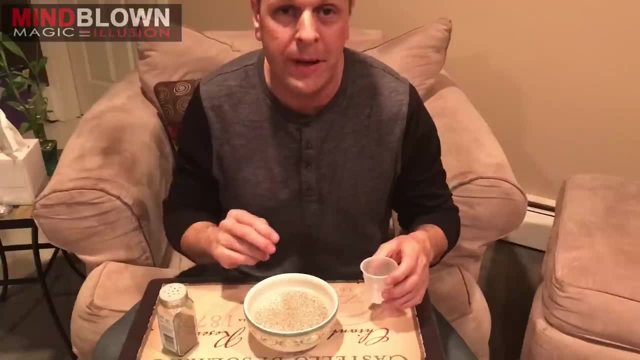 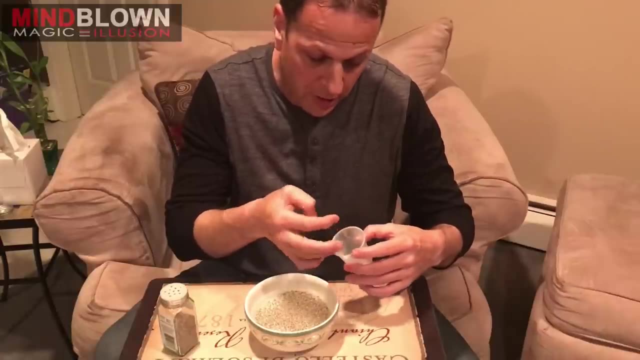 And then The secret is that there is a little bit of dish soap on his finger and I just have that in this cup. It's just regular dish soap that you'd wash your dishes with. You just get a little bit on the end of your finger. 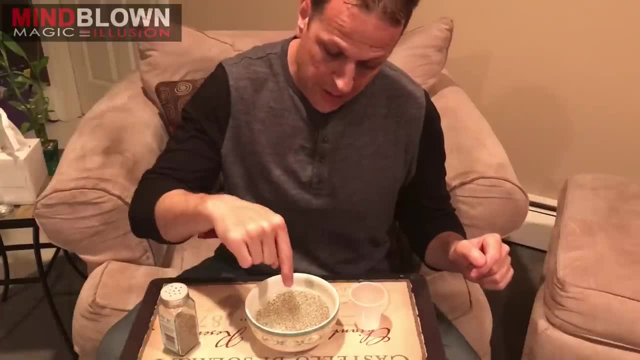 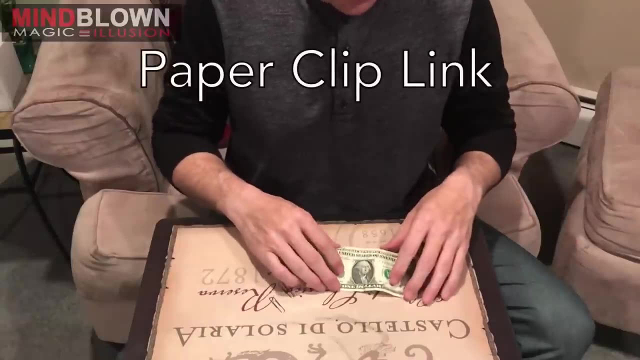 So now, when you make that magical gesture and you put your finger in the middle, the pepper automatically separates to the edges of the ball. This is another trick that really works by itself. All you have to do is place the paperclips in the right position. 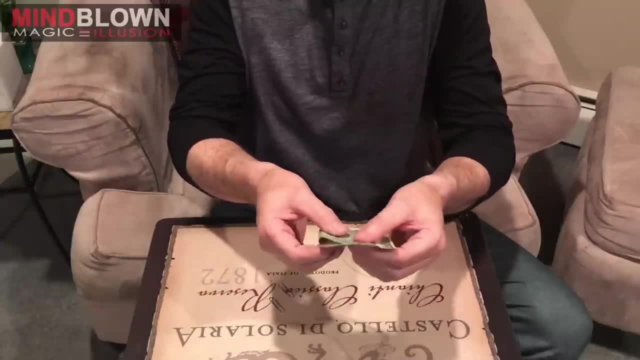 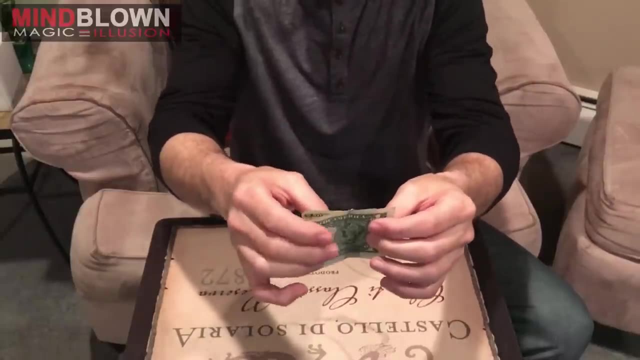 So what you'll do is fold the bill almost in half and put one of the paperclips right over both sides of the bill, Just like this. Then you'll fold this back the other way. take the other paperclip. 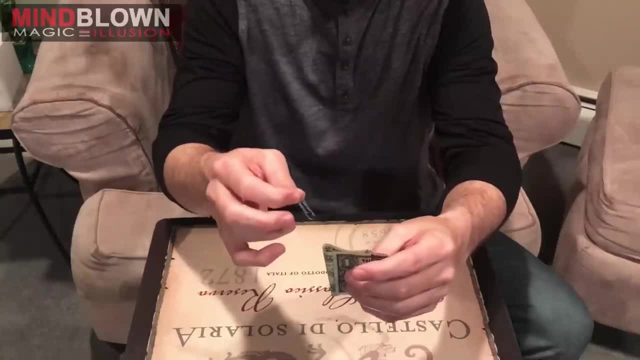 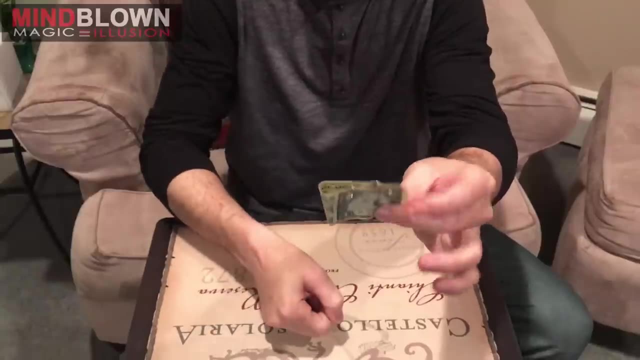 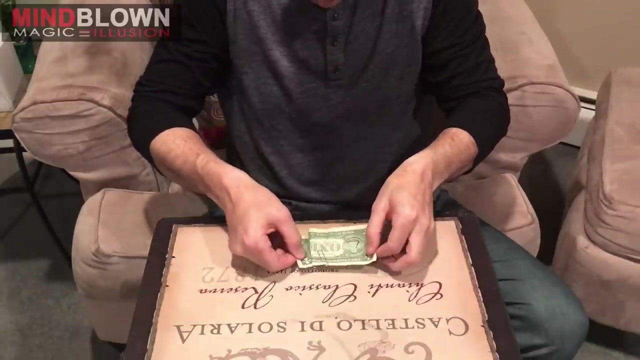 and you're not going to put it over the entire thing, You're only going to put it over the back two flaps Like this. Now, all you have to do is pull the two ends of the bill and they automatically link. 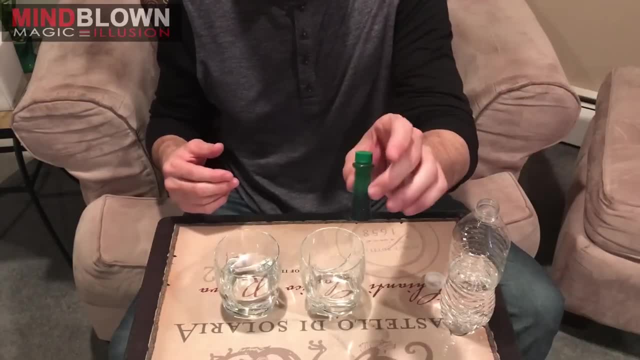 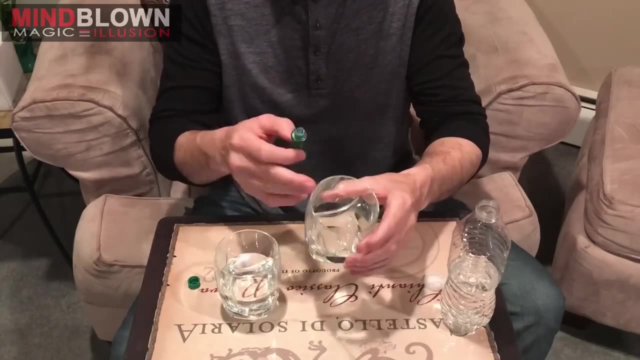 So the secret to the color changing water is food coloring, But it's important that you position it the right way so the audience doesn't see it. Now for the first part, I used two glasses. It helps to use a glass that has a little design in the bottom to hide the food dye. 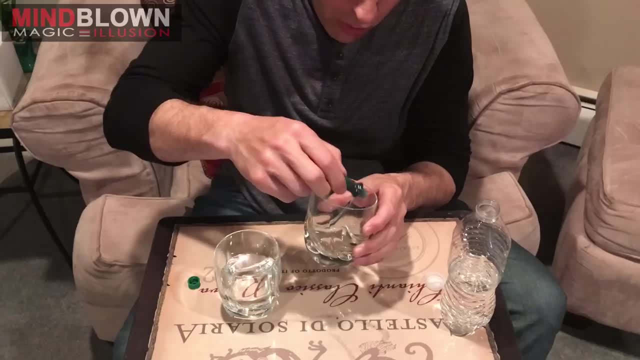 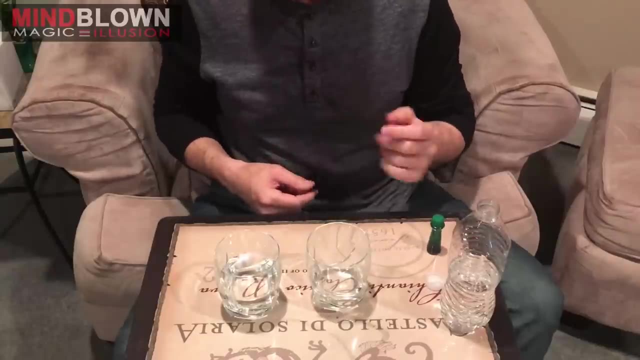 But all you do is put one tiny drop in the corner and now you have two options, Depending on where the audience is. they may not be able to see that, but if they can see it, you just hold the cup like this: 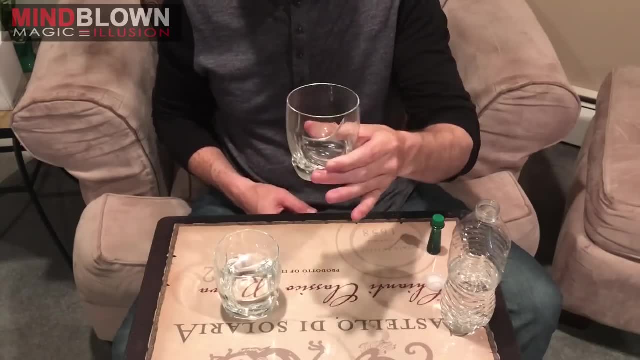 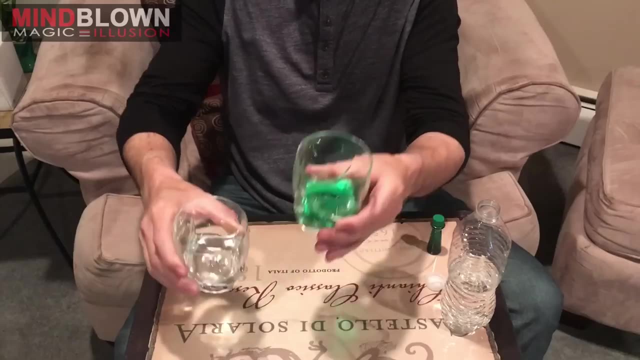 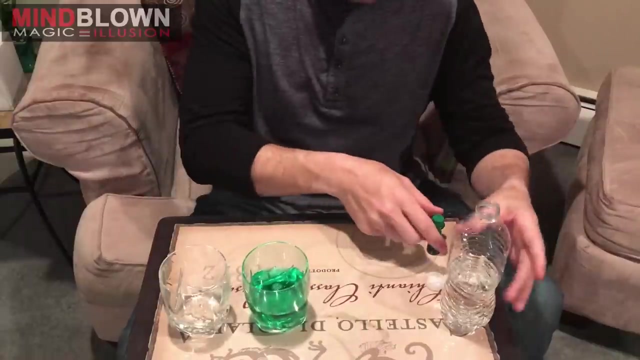 so you're blocking the food dye with your fingers. If you hold the cup like this, you just pour regular water in and as soon as it goes in it changes color. It's the same method for the bottle of water, except I put the dye inside the cap. 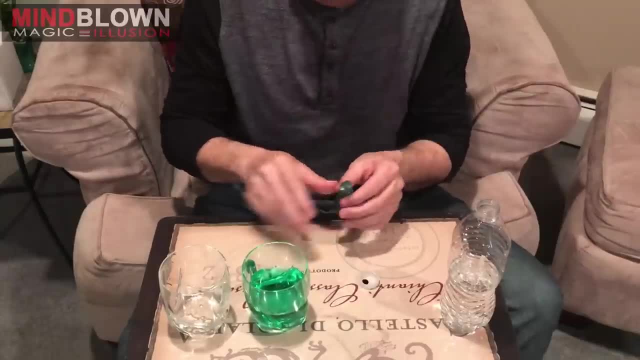 It's a little trickier here because you have to set it up way ahead of time. You need to let the dye dry so that it doesn't drip down. You don't want it to drip into the water as soon as you put the cap on. 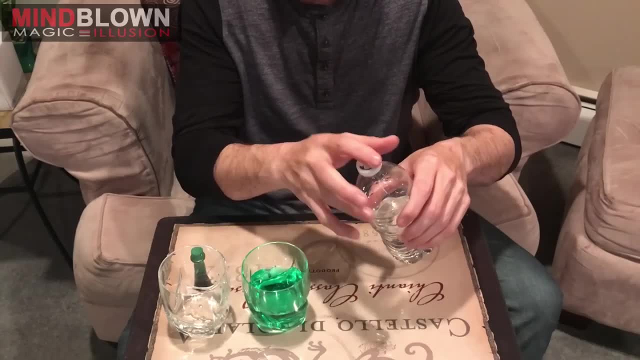 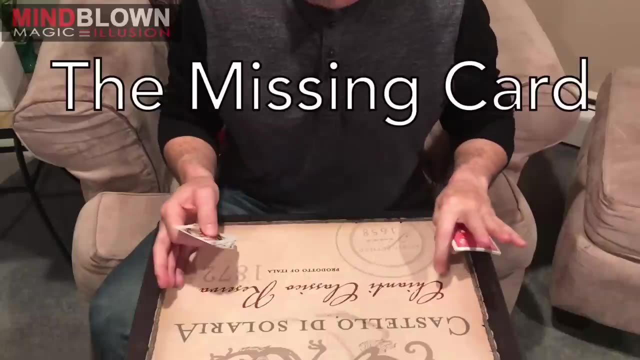 But the basic idea is: the cap goes on. you cover the cap with your hand and when you shake the water it changes color. This one is so much fun to perform and it always blows their mind, especially when a kid does the trick. 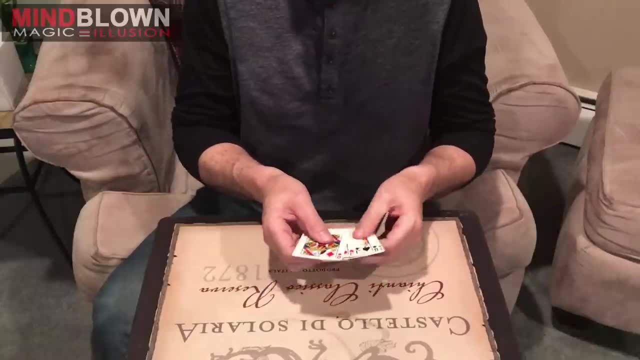 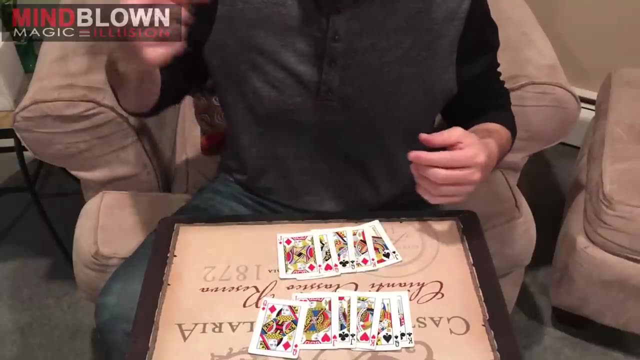 because parents don't expect what they've done. So here's how it works. We have a set of six cards, but we have another set of five cards behind the child's back or in their back pocket. Now they look very similar, but they're not the same cards. 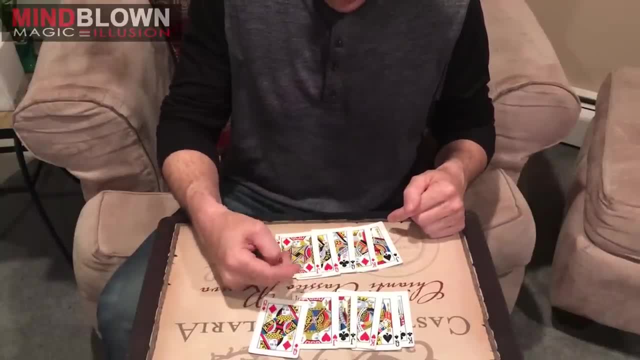 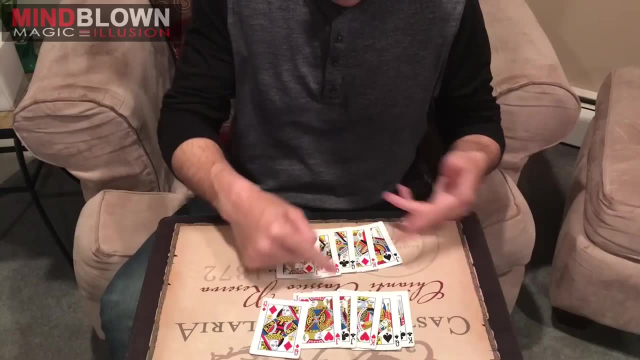 Every single one of these cards is different from these cards. So the Jack of Hearts is here, but the Jack of Diamonds is here, The Queen of Diamonds is here, but the Queen of Hearts is here, and so on. So all I've done is removed one card from here. 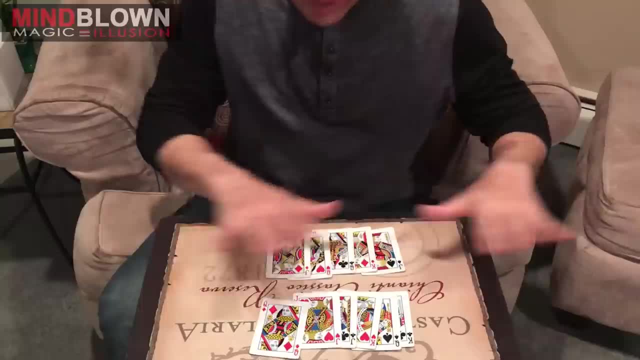 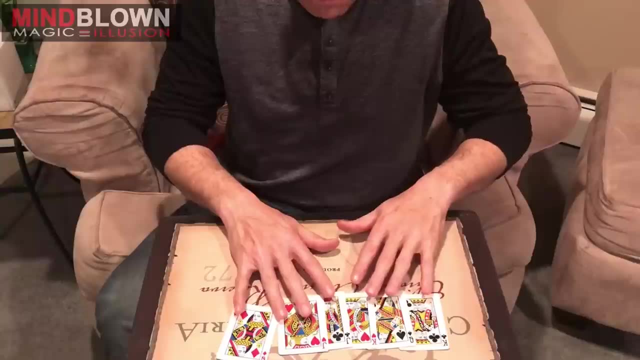 but it doesn't matter which card it is, because actually all of the cards are different. So, to begin the trick, the child would have these cards either in their back pocket or sitting behind them, and they're going to tell the spectator. think about one of these cards. 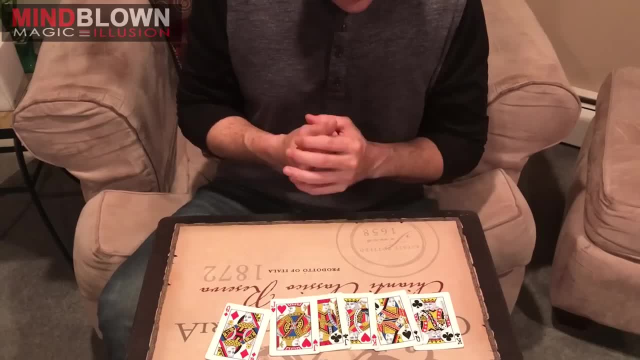 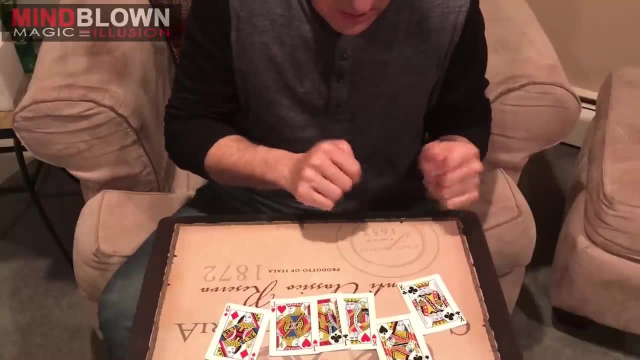 Pay attention to it. Remember that card. Now, what's great about that is the spectator is going to think of one card and not really pay attention to the other cards. So let's say they thought of the Queen of Spades- Great. So they're only thinking Queen of Spades. 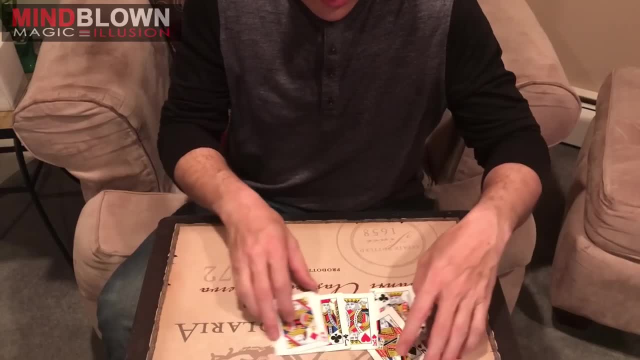 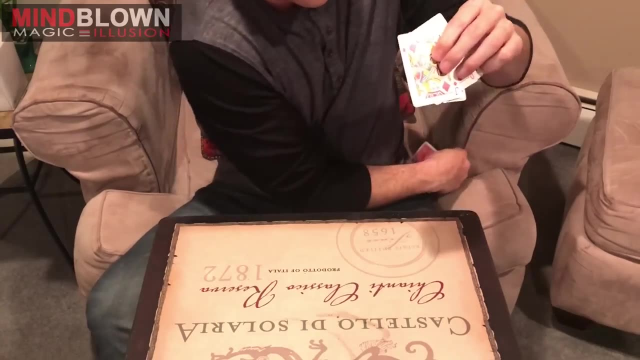 They're not looking at what else is there. Now the child puts this behind their back and all they're doing is swapping out for this bunch of cards while leaving this batch behind them, And when they show the cards, of course, that card is gone.